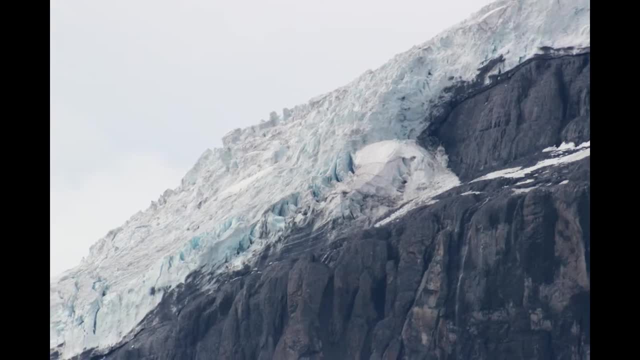 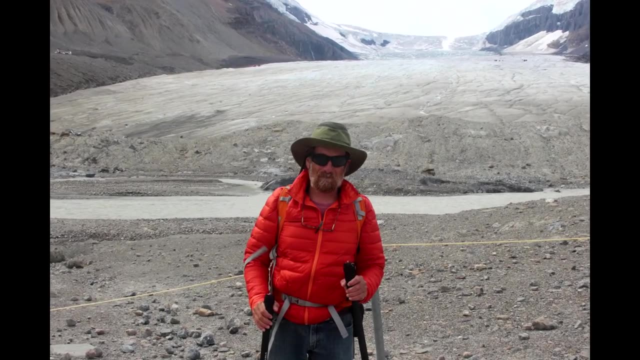 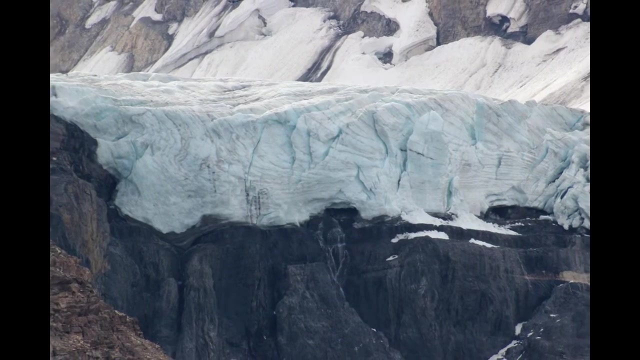 it covers the ground and the next snow falls on top. As the snows get thicker, it weighs down on the snow below and packs it tighter and tighter. Eventually, you end up with a thick, strong matrix of ice that we either call a glacier. 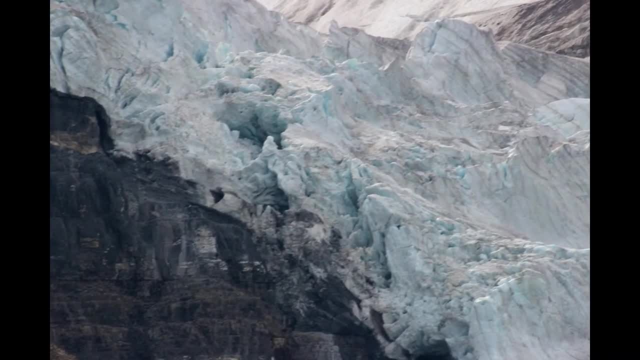 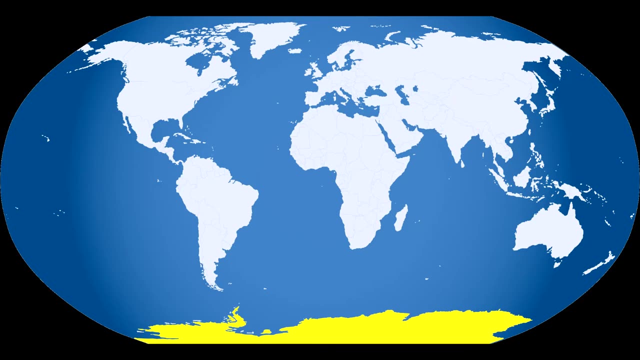 or an ice sheet. What's the difference? Mainly size. The massive ice sheet that covers Antarctica or the one that covers Greenland can be two miles thick. in some places The ice sheet covers thousands of square miles. That's an ice sheet. Glaciers are much smaller. 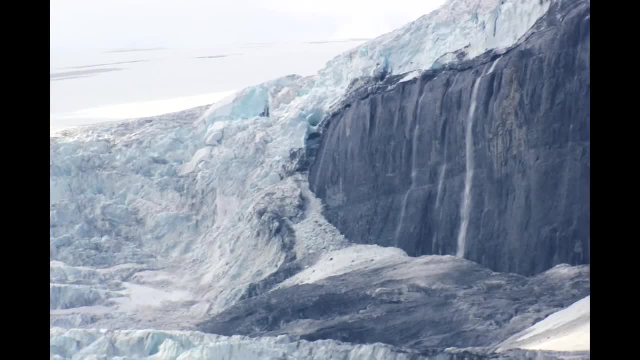 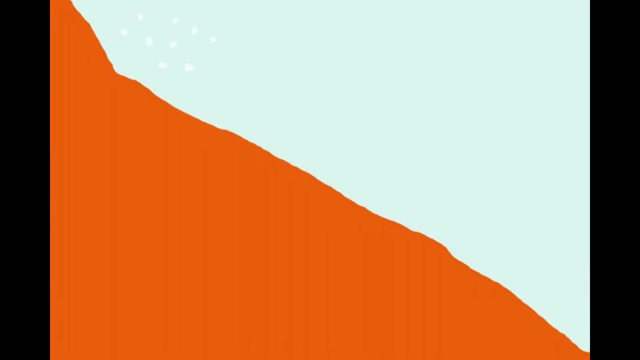 like these alpine glaciers in the Canadian Rockies, Glaciers and ice sheets are complicated structures. As snow continues to fall on ice sheets and glaciers, the glacier is squeezed out on the sides and pushed along the continent or mountain where it forms Eventually the 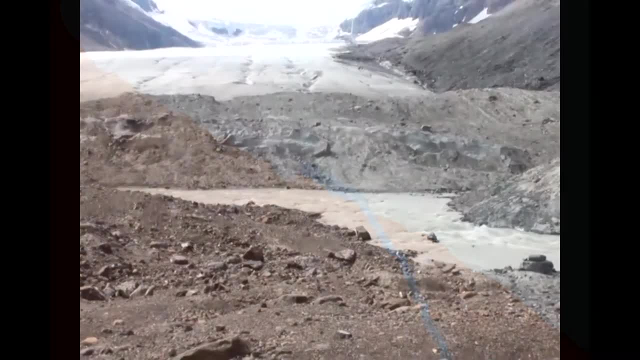 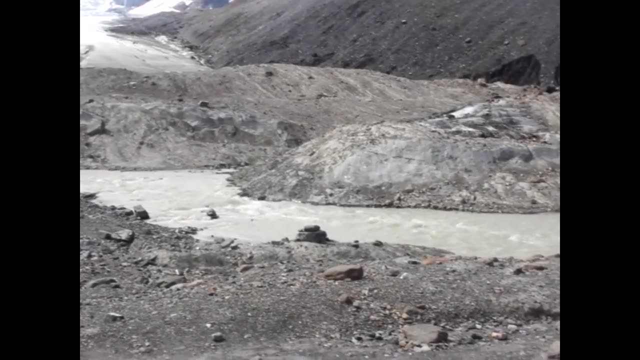 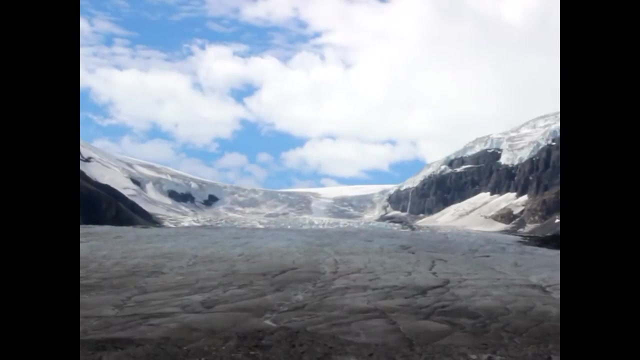 end of the glacier travels along until it reaches a point where it finds warmer areas and melts too quickly to continue building up. That's the edge of the glacier, or ice sheet. The edge of the glacier will melt while snow and ice continue to build at the center. 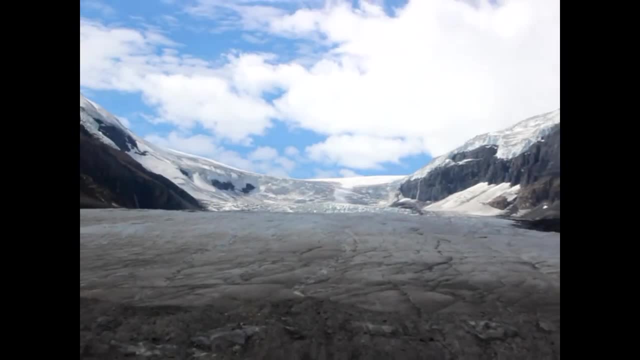 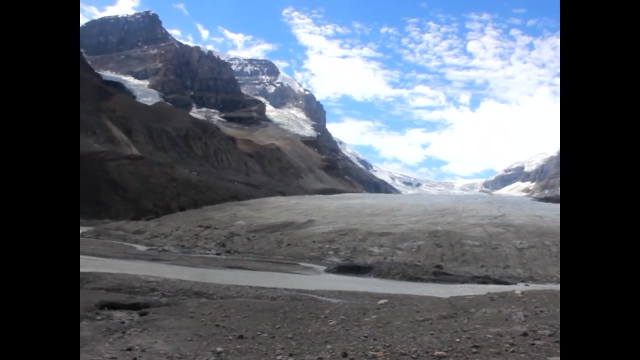 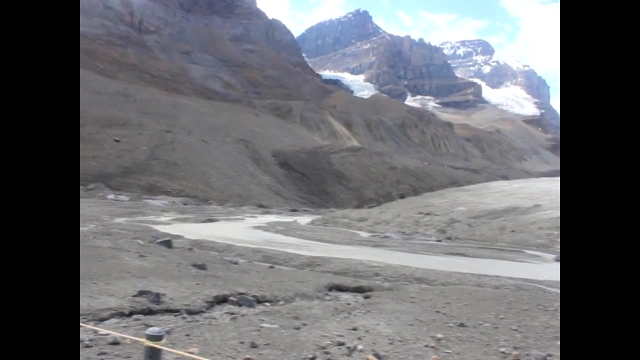 Glaciers, ice sheets and even sea ice all actually move very slowly as the ice makes its way around from the top to the bottom or the center to the edge. Have you ever heard the expression at a glacial pace? It means really, really slowly, and now you know why. 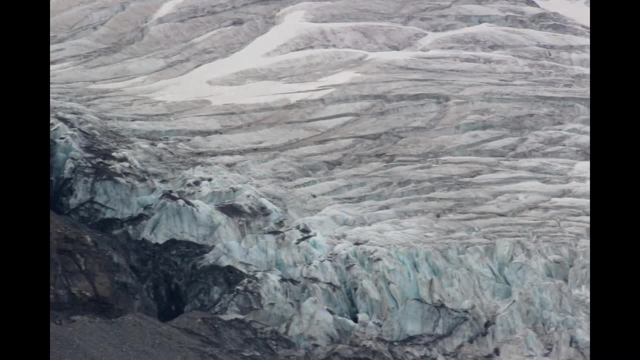 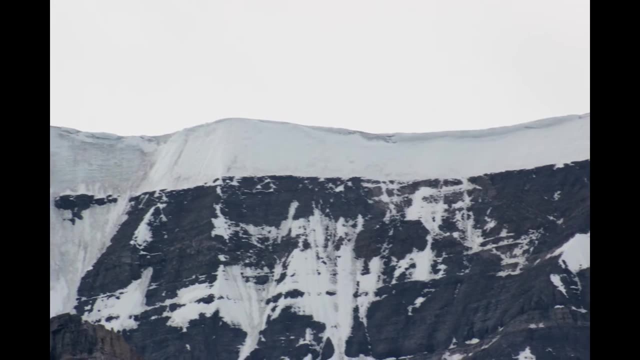 Are glaciers. important Climatologists call them the air conditioners of the planet. Air that travels over ice in the far north, or even in the mountains, gets cool very quickly, and when it collides with warmer air from the tropics, that temperature difference. 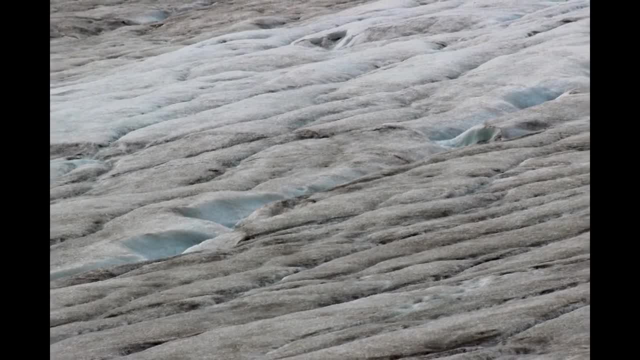 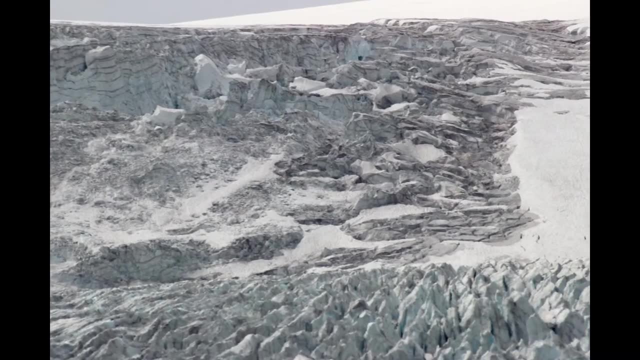 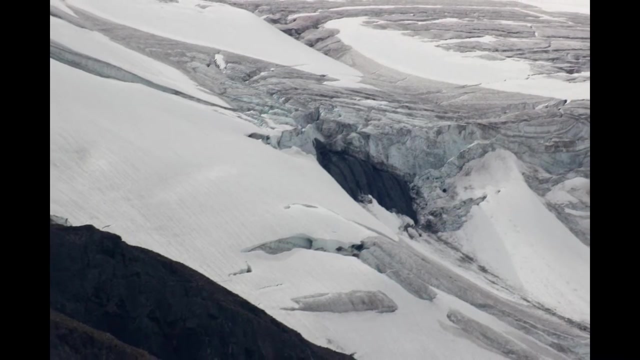 helps create the weather and climate. our bodies are adapted to survive in What happens as our climate warms. Well, as you might imagine, snow and ice melt All over the world. the cryosphere is getting smaller. Alpine glaciers like this one are.